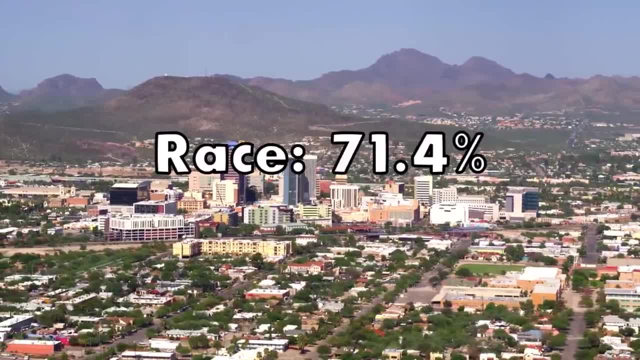 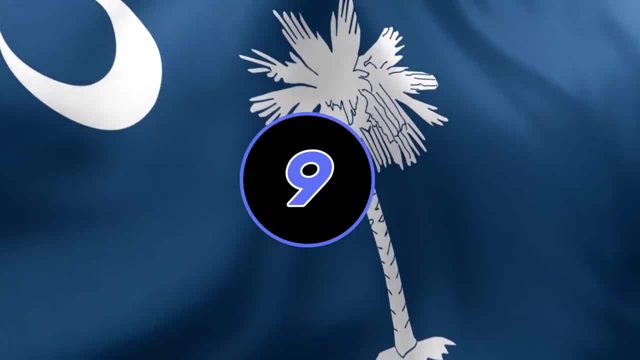 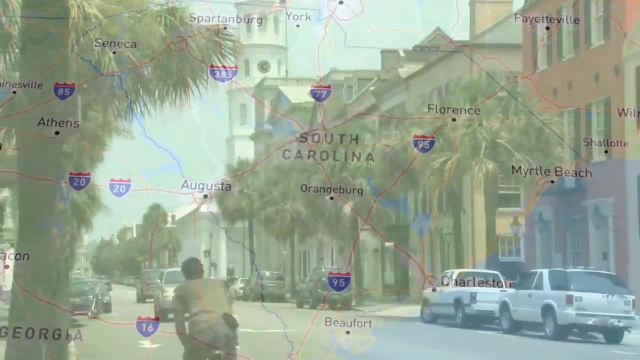 culture and the state government. In Arizona, 71.4% of their bias-motivated crimes are towards race, ethnicity or ancestry. Number nine: South Carolina. South Carolina has a long troubled history when it comes to race relations, including a history of slavery and segregation. The state has also been criticized in recent years. 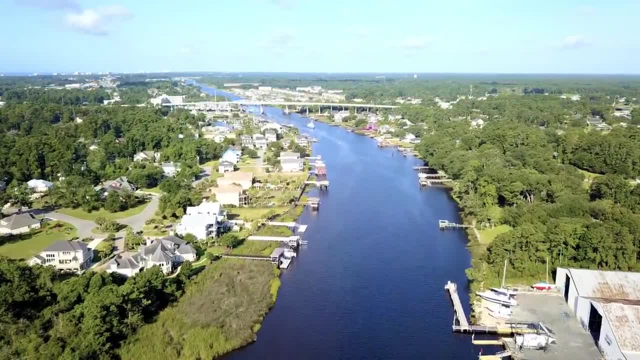 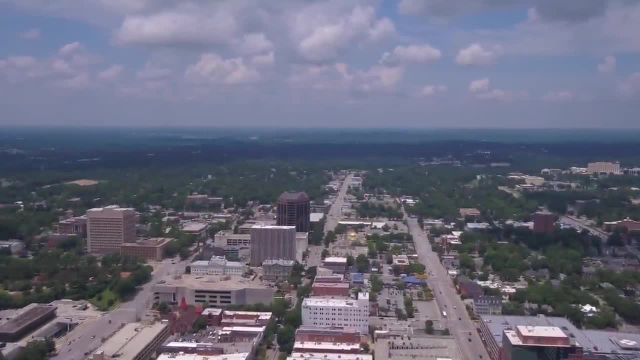 for voter suppression efforts. I mean, they've had that for a while, but it's coming back in the news again. They've been trying to purge voter rolls and a whole bunch of other things In 2022, they went back in the news with a new voting law which many argue will disproportionately affect. 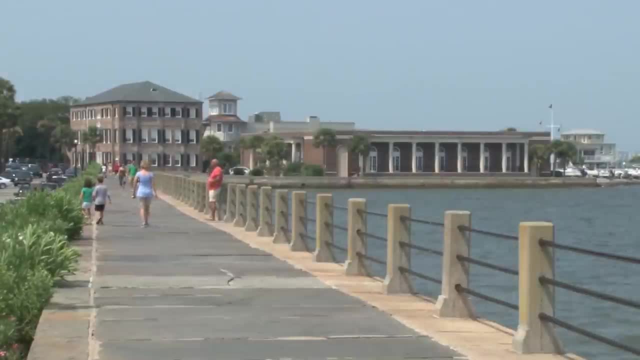 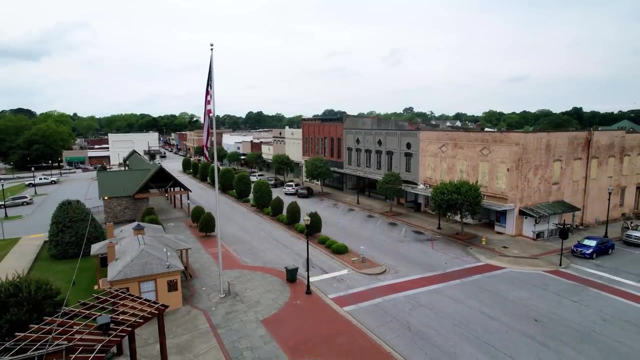 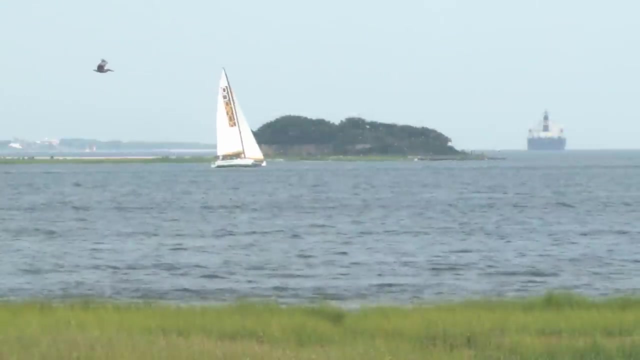 people of color. When it comes to bias-motivated crimes in South Carolina, it's not always about race or ancestry. They go after each other for religion and sexual orientation. 28% of those crimes are against people of another religion And sexual orientation is about 11%. South Carolina is one of those states that nobody 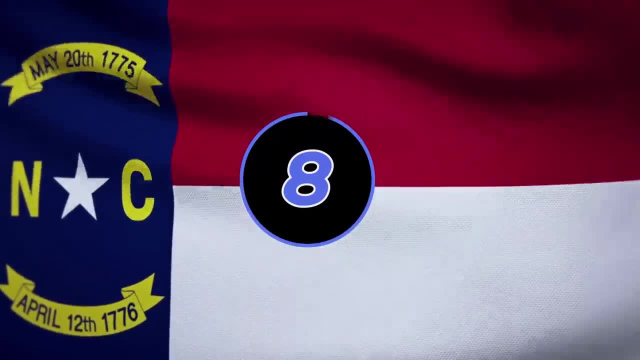 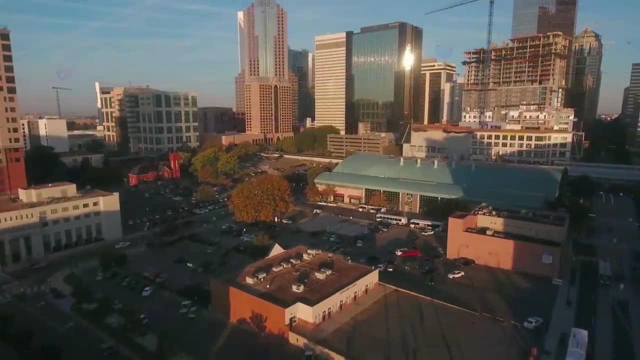 should be surprised by Number eight, North Carolina. North Carolina has a history of discrimination against African-Americans, particularly in the voting rights. Now you'll see voting rights here a lot. That always seems to be the go-to thing when you're looking. 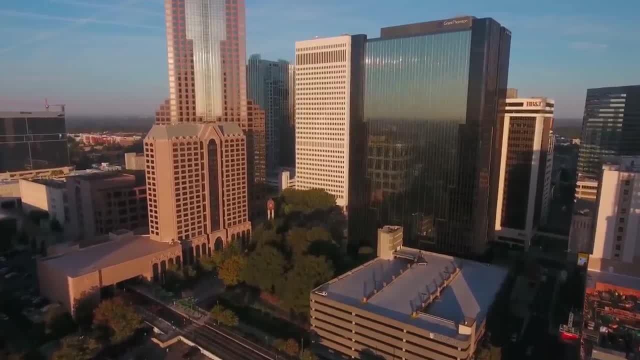 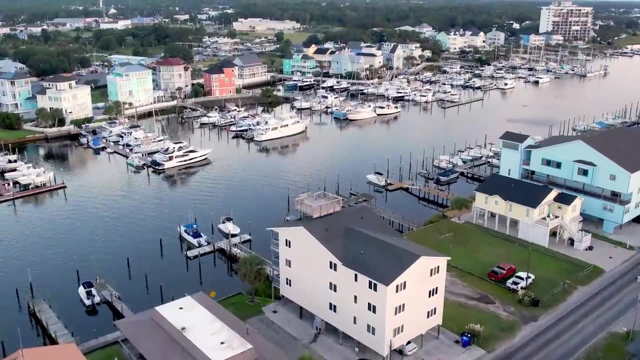 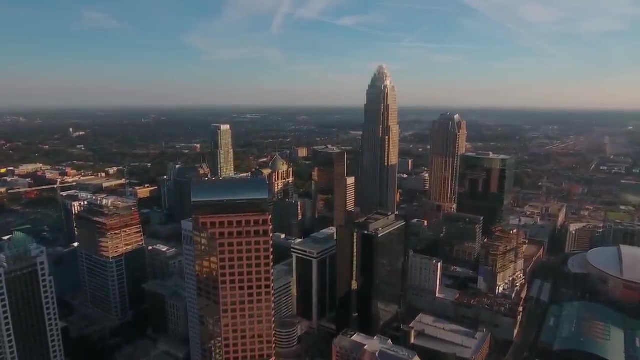 at racism in different states, But North Carolina has been criticized for voter suppression efforts, which include strict voter ID law and purging of voter rolls. They're another one that's been in the news in recent years, with stricter voting laws. Now we know we do have to have voting laws and I think there should be an. 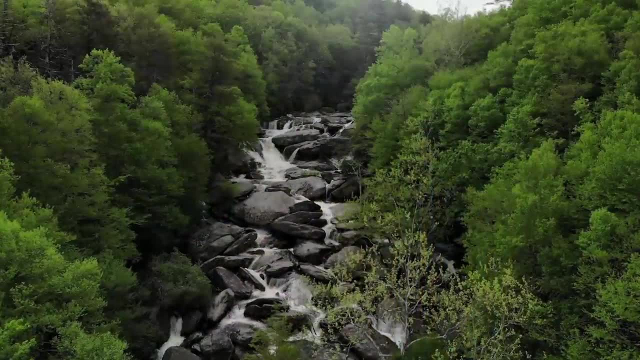 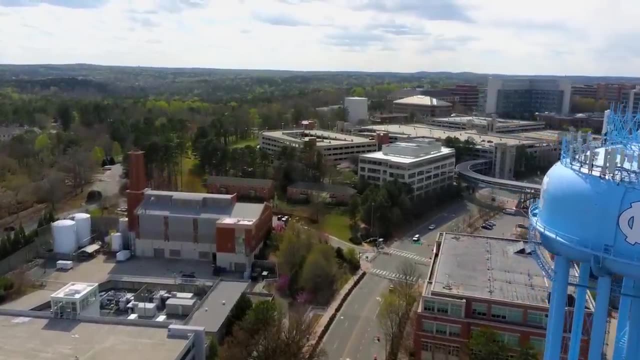 ID with it. But I think if they're going to make that ID, they got to make it easy to get to, like at every city hall or something like that. One of the biggest problems that people have with that voter ID thing is if you want to get it done, there's some hoops you got to go through. And a lot of times you got to go to some office that's like 20 miles away or something and obviously they feel it's targeting people living in poverty who don't have the means to just drive around to some office and wait three hours while you get some government official to. 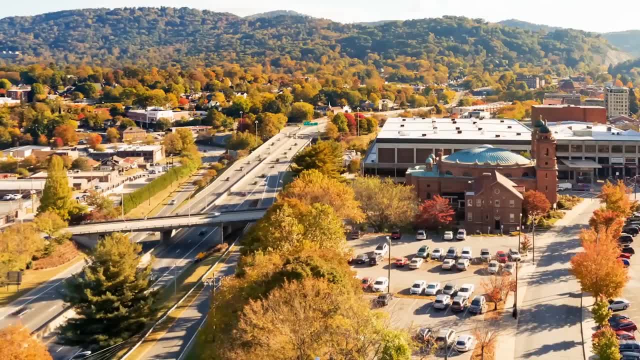 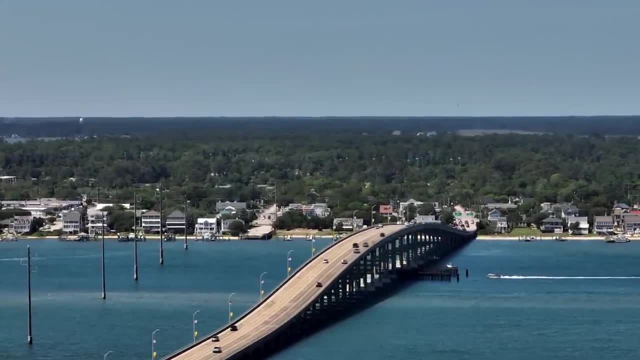 give you a voter ID Just as long as we don't go to that thing that they have in some Central American countries where you vote and then they dip your thumb in like this ink that doesn't wash off for like a week or a month or whatever, So they know you voted. So if you show up at a place, 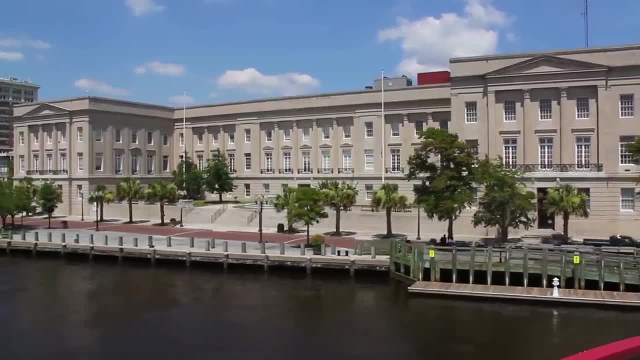 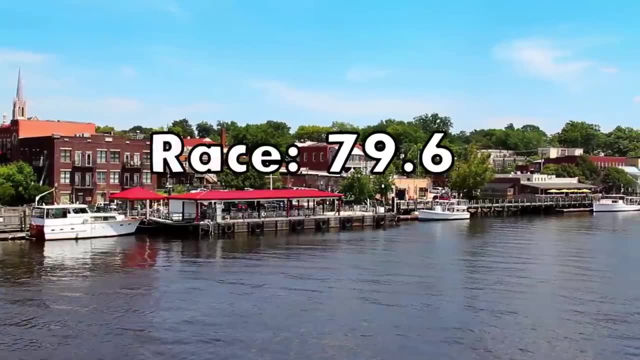 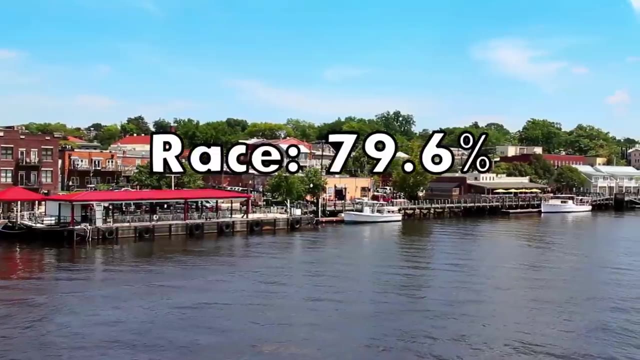 to vote. they always got to look at, like your left thumb, to see if it's been dyed or not. That might be good. Then people quit wearing those stupid stickers. I voted as they get their latte. 79.6% of North Carolina's bias motivated crimes are race and ancestry related. 13.4%. 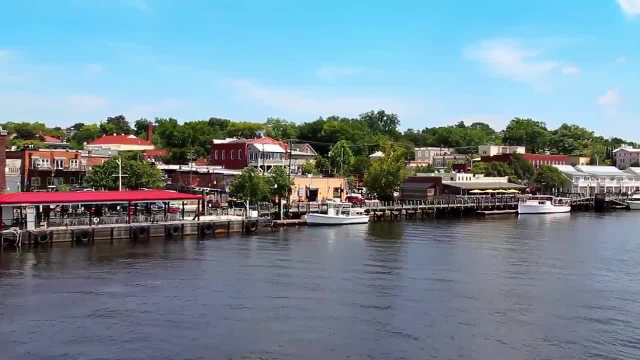 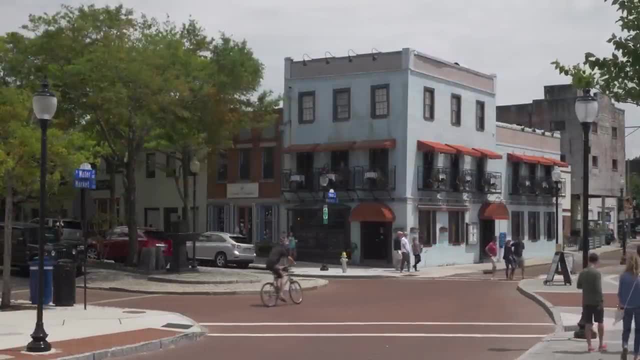 are sexual orientated and religion is 6.5%. I think North Carolina is another state where they've got some good sized cities And I don't think a lot of the people there really care about the gender thing or gender identity. It's just not how North Carolina is. Number seven: Texas. Texas has a large, diverse population, but it still faces significant issues when it comes to race relations. The state has been criticized for its harsh immigration laws which, like Arizona, many feel are rooted in the local government and the culture of the people. 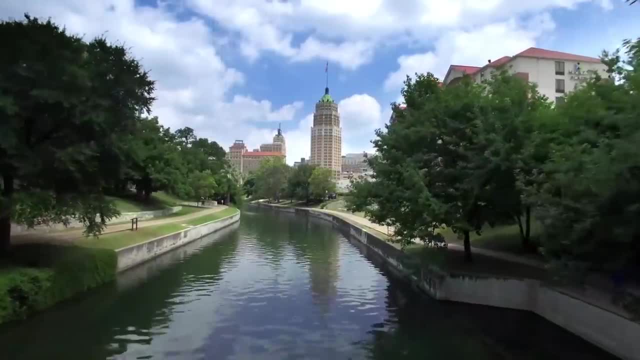 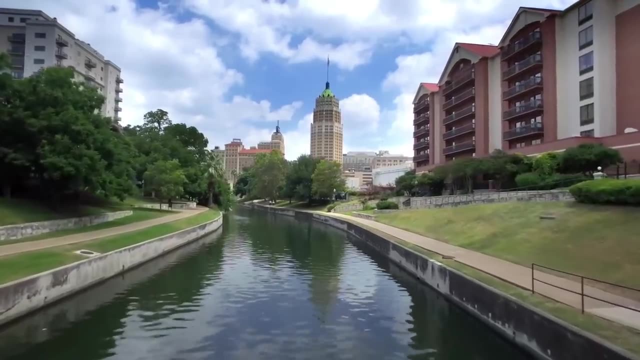 Now this one. I don't agree with this one And it's just from my experience. I'm sure you can have all kinds of stories where there's been racism in Texas, but that can be everywhere. But my experience with people from Texas 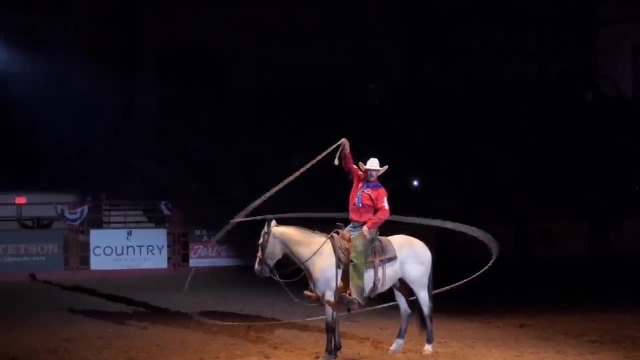 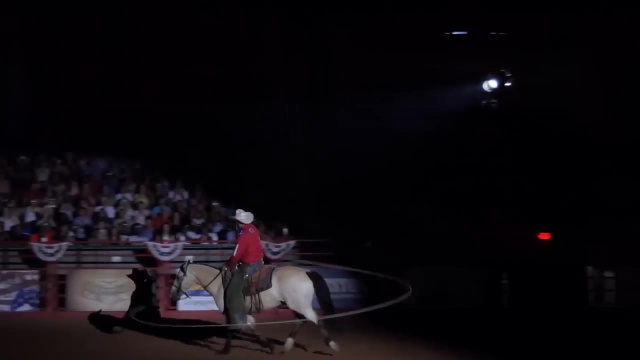 when I've been in Texas, there really wasn't much of it. That's just my own thing, And sometimes your feelings don't match up with the stats. In this case, that's my views of Texas. Texas also has recently tried to pass some new voting laws which again, many argue disproportionately affect. 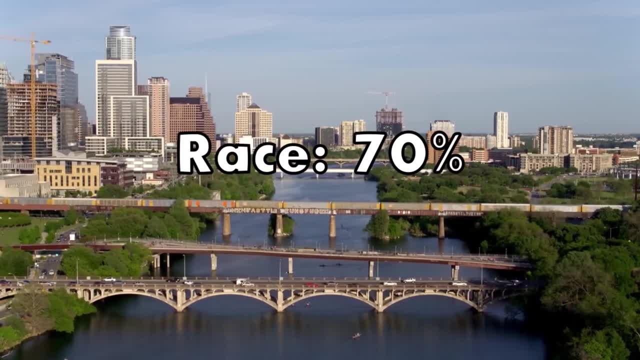 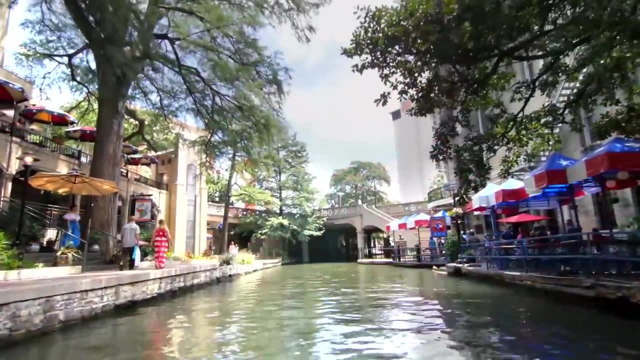 people of color. Now, when you look at bias motivated crimes in Texas, 70.1% are due to race, ethnicity and ancestry. You know I'm having a really hard time saying ethnicity today, so I'm just going to drop it. 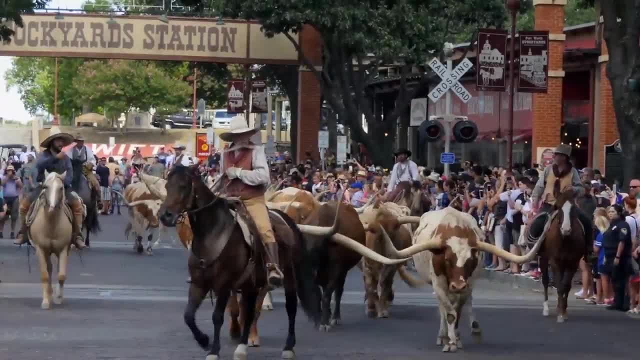 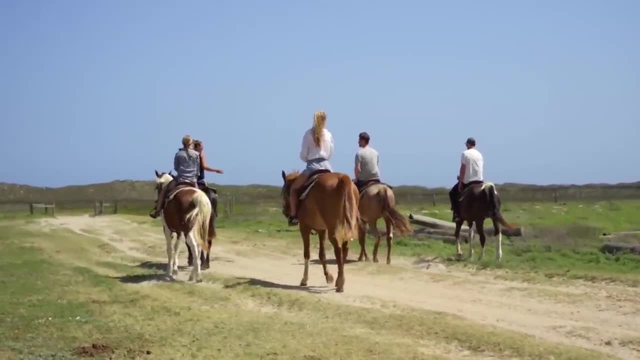 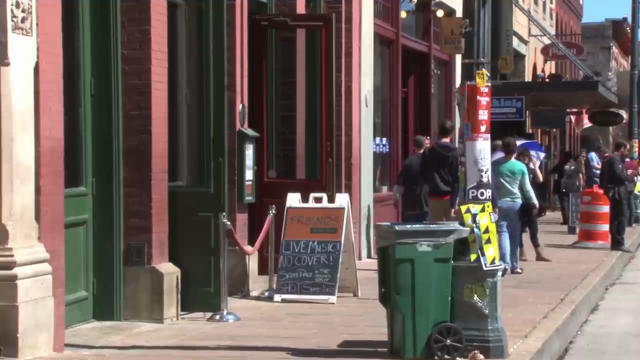 Just let it be known. I mean it also in all of them, but 17% are because of sexual orientation and only 7.5 are because of religion. Now here's a new one that's growing in Texas: gender identity. That's 1.9% of the bias motivated crimes, And that, of course, is 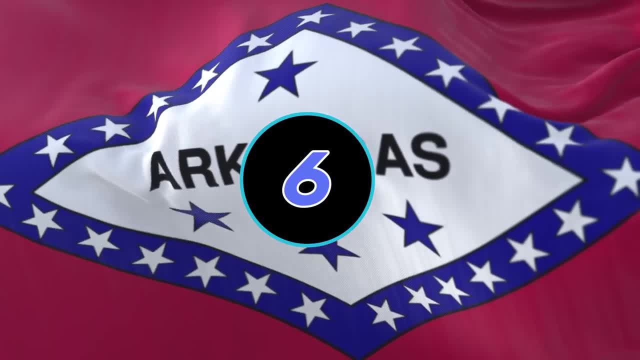 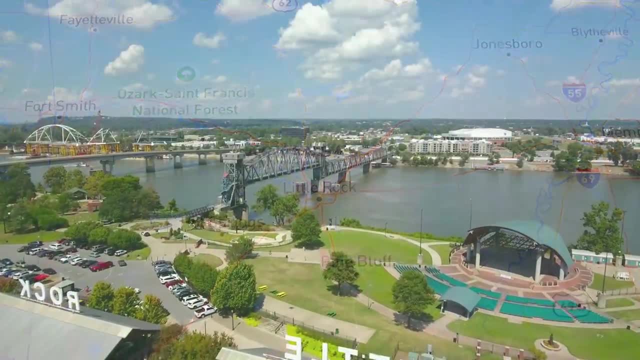 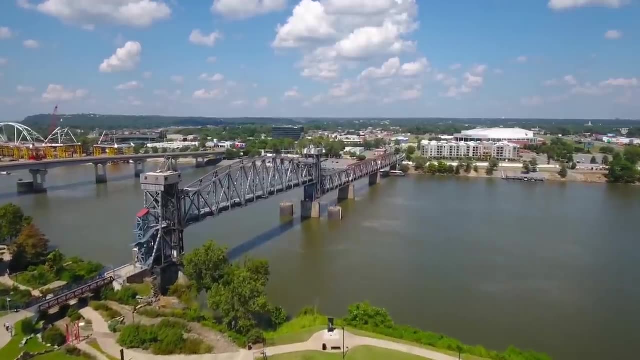 according to the department of justice, Number six: Arkansas. surprise, surprise. Our old pal Arkansas shows up on a list like this. This one should be no surprise to anyone. Arkansas has a history of segregation and discrimination, especially when it comes to education. The state has been criticized for its underfunded and 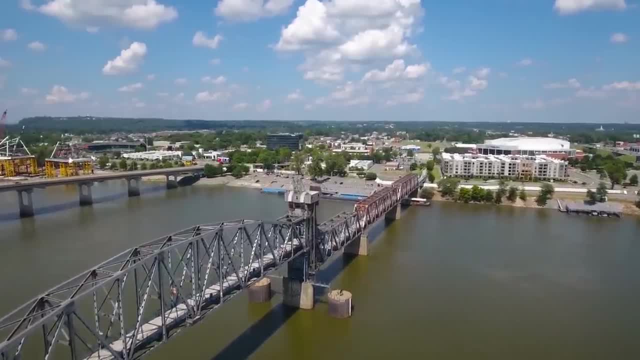 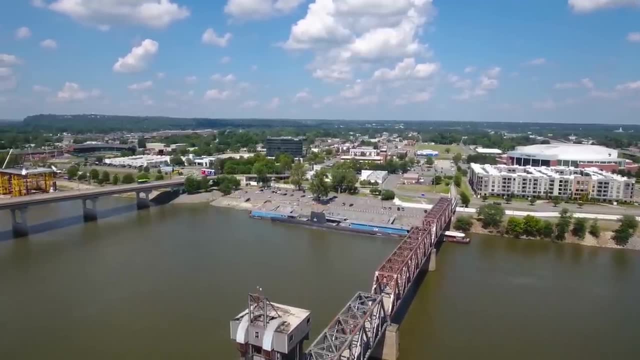 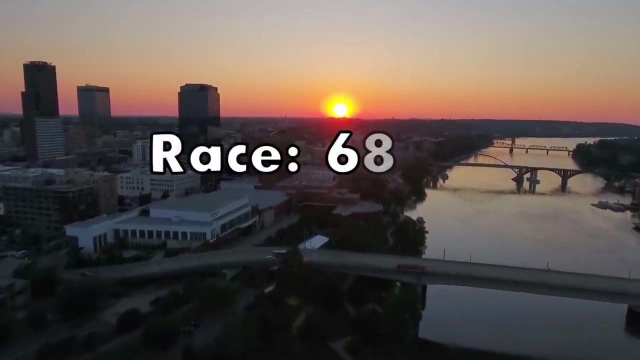 segregated schools, which have contributed to persistent racial achievement gaps. Arkansas is another one of our fine States That's been accused of voter suppression efforts. Now, according to the department of justice, their bias motivated crimes look like this: race and ancestry are 68.4%. Sexual orientation is 21%. 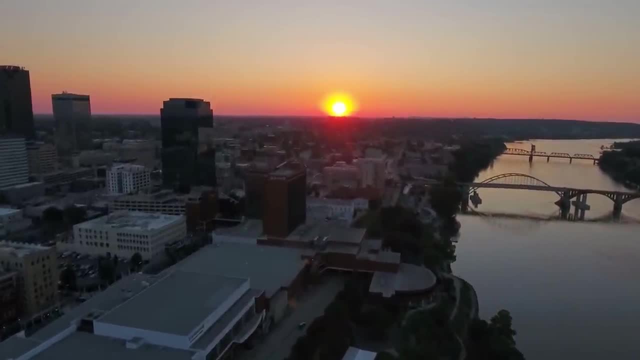 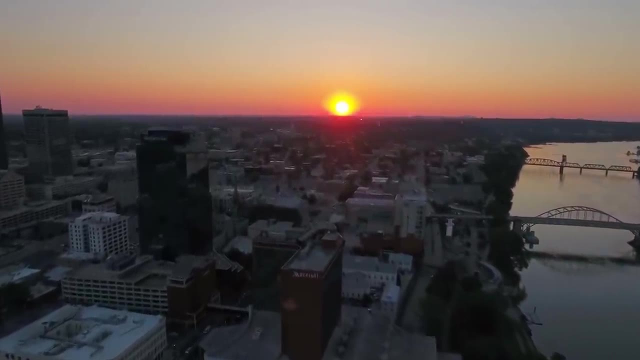 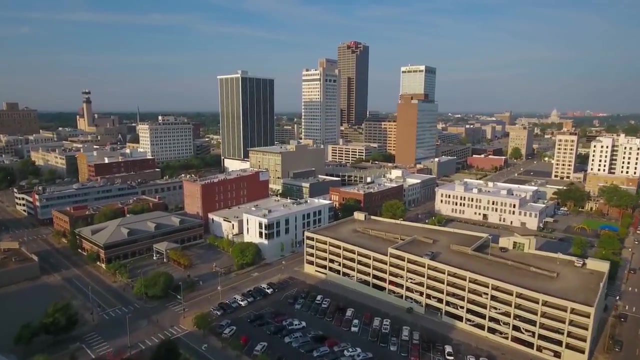 1.1% Now they have no problem. It- at least it appears on these numbers here with gender identity is zero. They don't have many crimes like that, but when it comes to religion, yeah, they do. It's actually 11% myself. I think the reason they don't have many gender identity 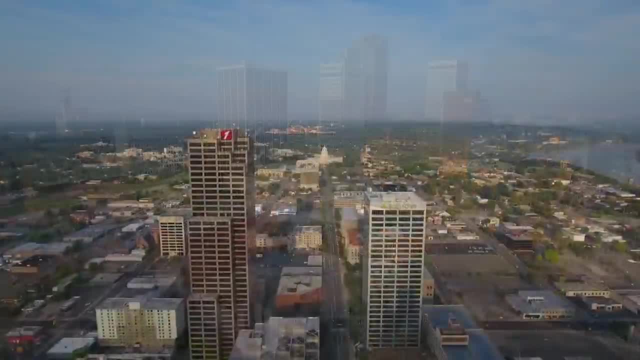 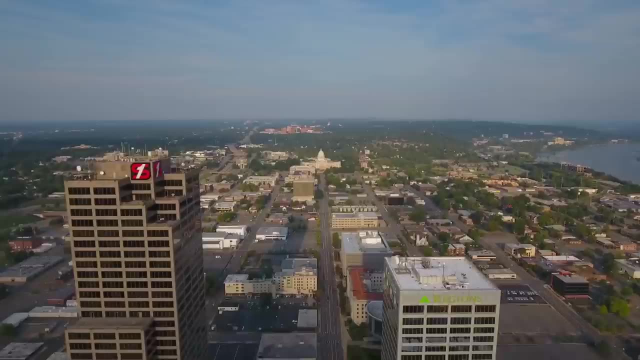 motivated crimes is because people that are transgender probably know not to go to Arkansas. Now this whole video is kind of based on race and ancestry- I mean the most racist States, but this kind of flows into it all the bias motivated crimes. Now there's a reason I have 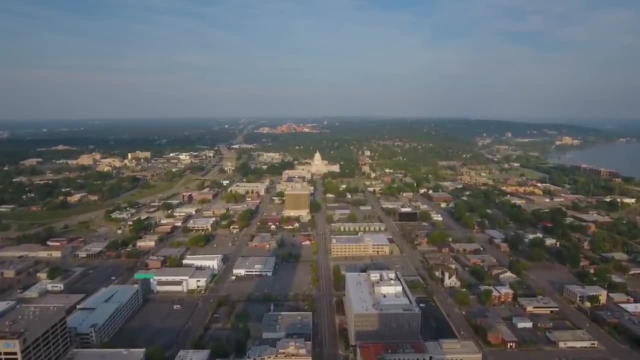 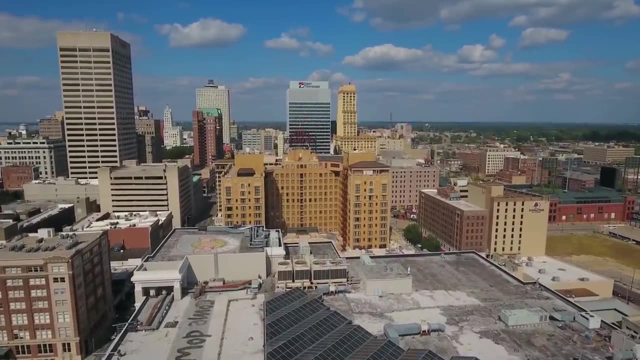 to say that if I leave that door open, you're going to have a bunch of jackaloons in the comment section going. when did transgender become a race? When did sexual orientation become a race? This video is about race. I've been doing this a long time. I kind of know when I'm leaving the door. 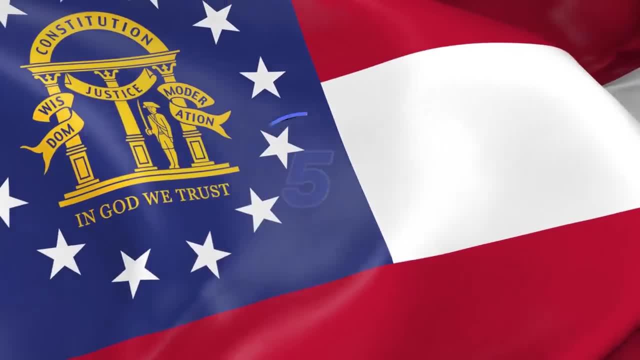 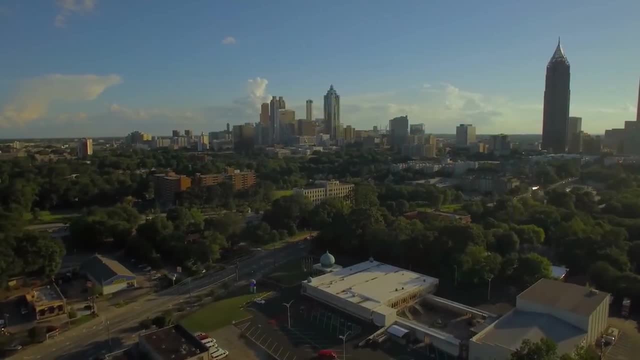 open for people. Number five: Georgia. Now, in my opinion, I think Georgia is one of the States That's made the most improvement since, let's say, the 1950s, Especially when it comes to the Southern States. Georgia has a long history of discrimination. 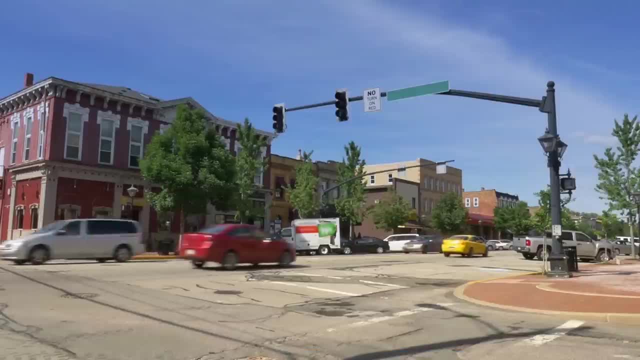 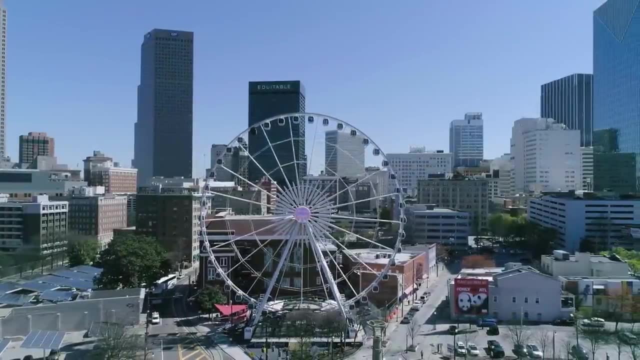 against African-Americans dating back to the days of slavery. The state has been criticized for voter suppression efforts, which includes strict voter ID laws and purging of the voter rolls, And, of course, this was brought up in the news during the 2020 election. whole bunch of political. 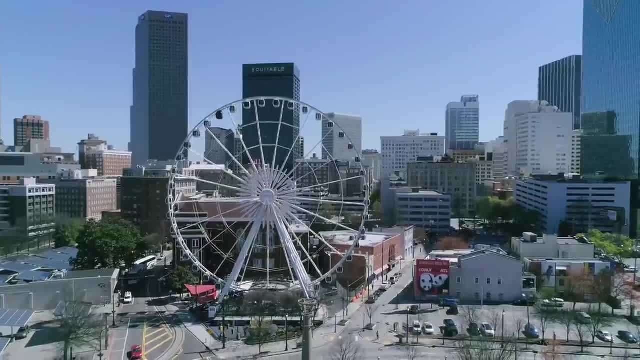 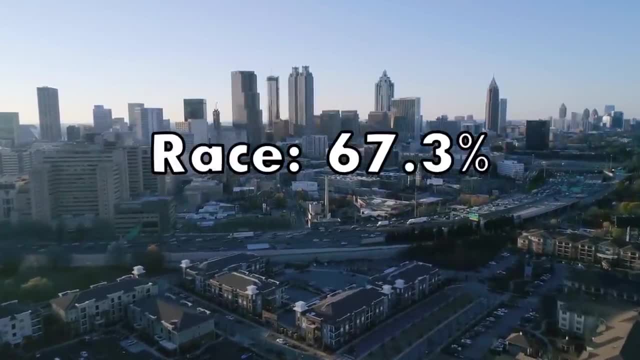 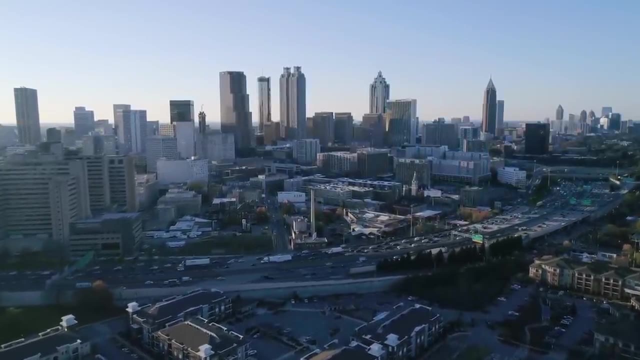 nonsense was going on in Georgia And this was part of it. Now, according to the justice department, Georgia has its other issues. Let's look at their numbers for bias motivated crimes, 67.3% of those are because of race or ancestry. Religion is 13.3%. Sexual orientation is 12.2%. Here's a new one. 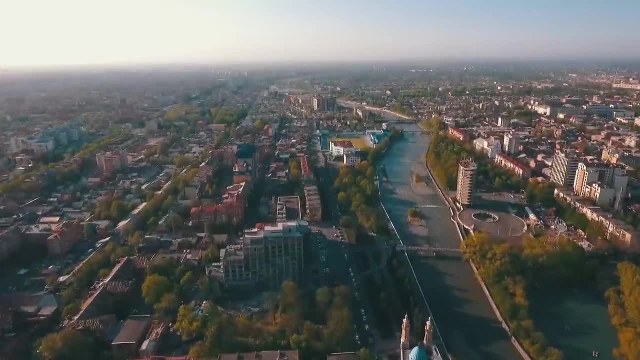 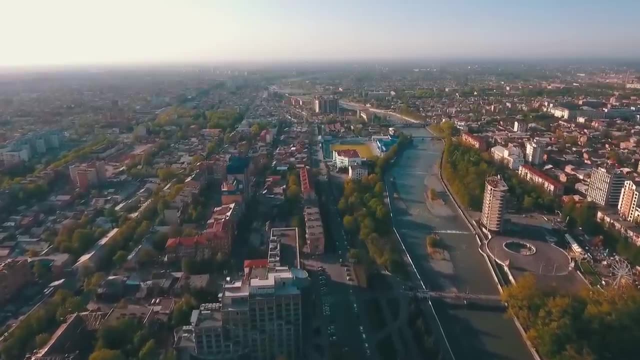 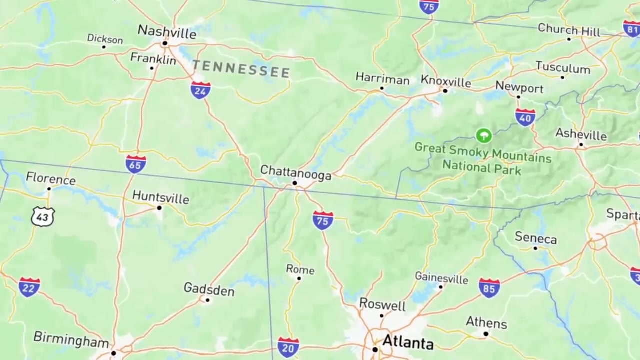 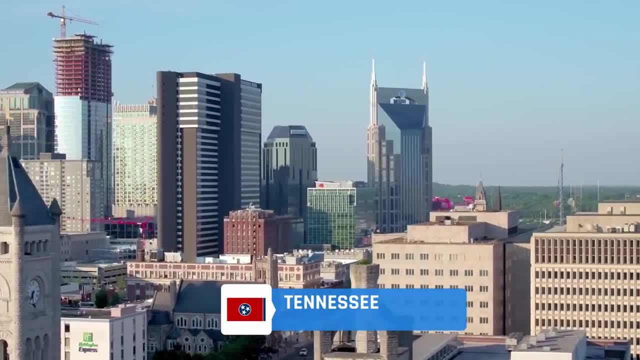 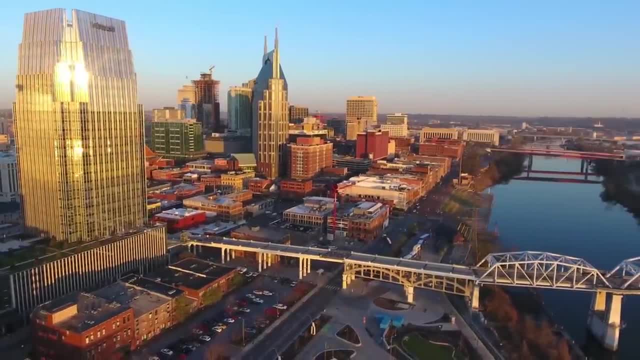 reflect on the people I know from Tennessee and I really don't see much of this in them. You know 10, 15 people. it's not a good sample size, but that's just kind of my opinion. That being said, 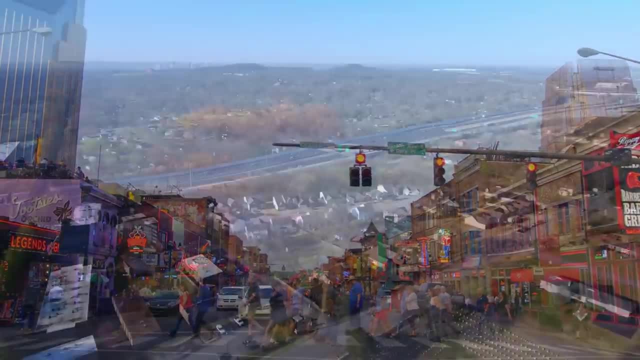 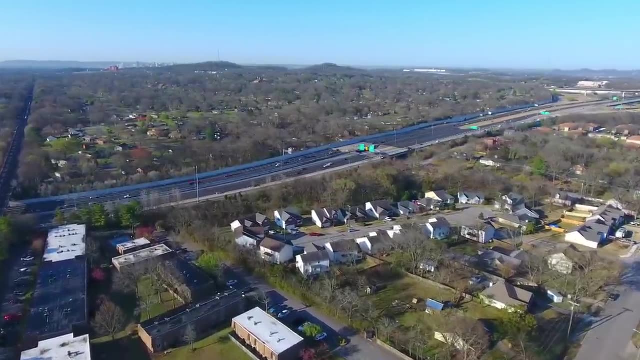 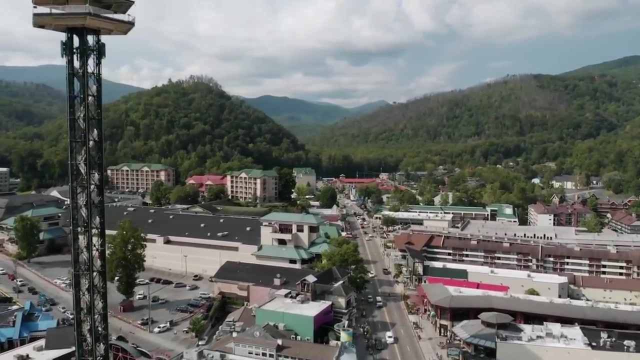 the volunteer state has a history of racial discrimination And again, especially when it comes to education, the state has been criticized for underfunded and segregated schools. This of course means fewer minorities going to college, less college attainment, a smaller educated workforce, And this just kind of keeps the state where it is: A lot of poverty. 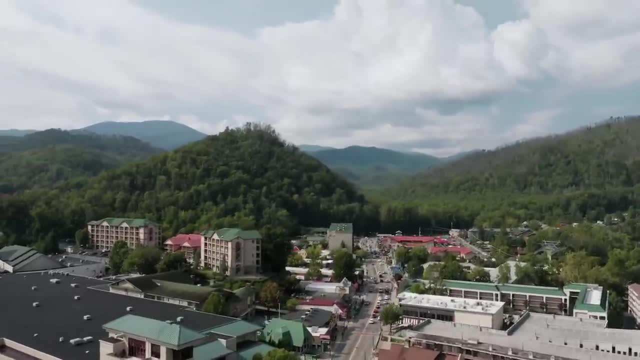 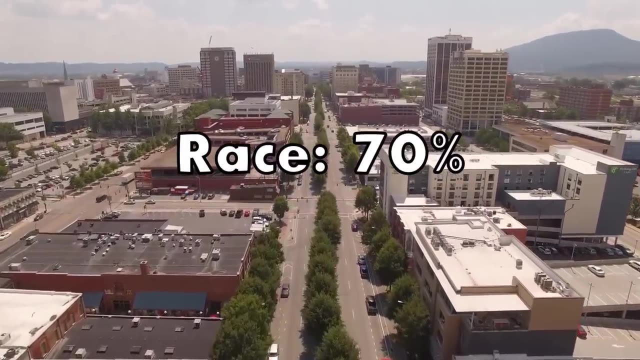 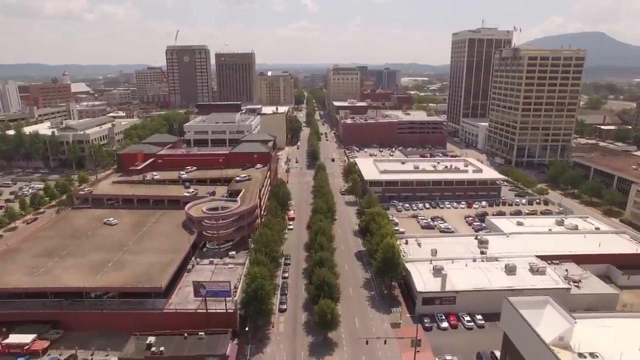 Tennessee also has a history of voter suppression and disenfranchising people of color. When it comes to bias motivated crimes in Tennessee, 70% of them are race or ancestry, with 20% being sexual orientation. Religion comes in 5% of them and gender identity is 2.5.. Number three: 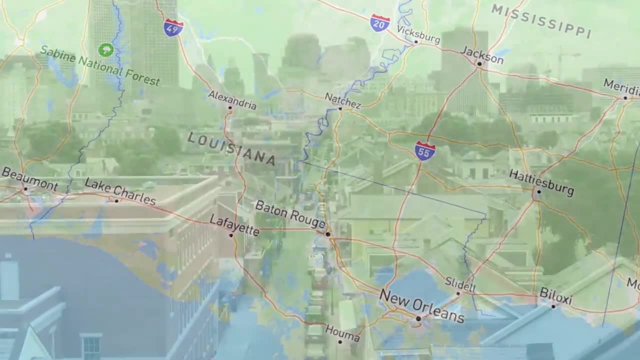 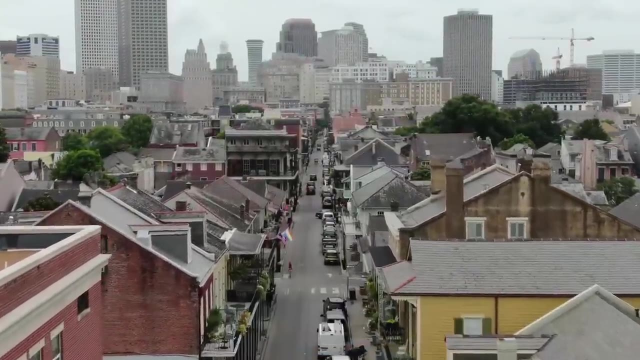 Louisiana. Louisiana is another state that has a very difficult history when it comes to race relations. The state has a high percentage of African-Americans, but they still face significant discrimination in areas such as employment and housing. Louisiana also has one of the harshest. 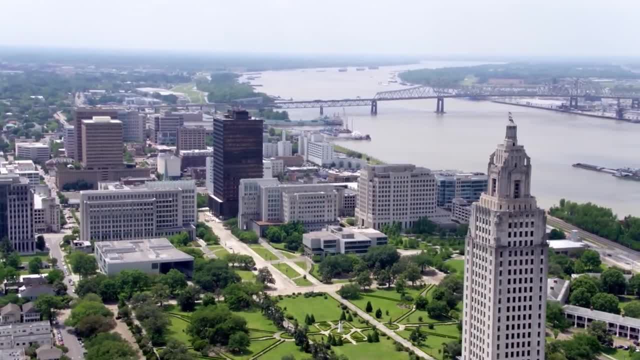 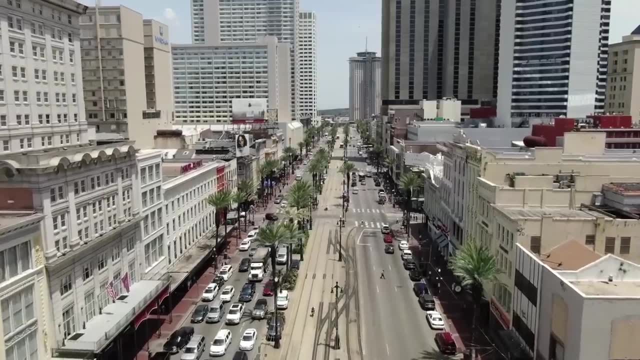 criminal justice systems which really leans into people of color. Louisiana is another one of those states where you're going. yeah, no kidding, When it comes to bias, motivated crimes, race and ancestry is 67.5% of those. So it's a very difficult state to live in And it's a very difficult state. 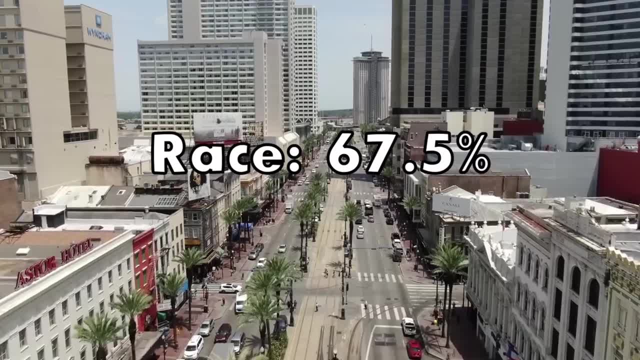 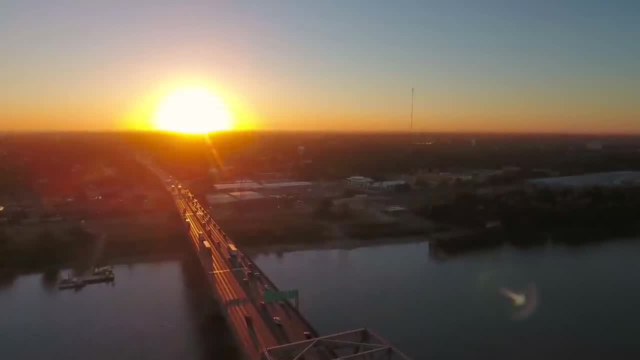 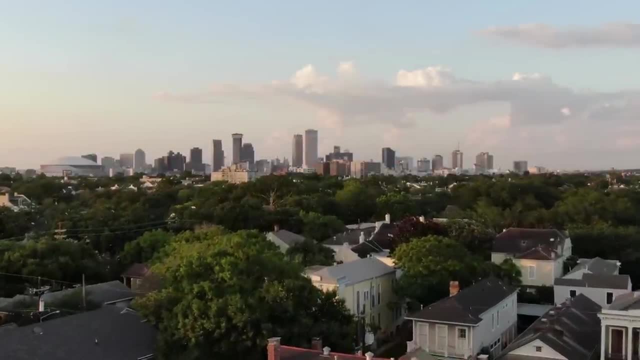 sexual orientation is 15%, Religion is 12.5% and disabilities is 2.5%- well above the under 1% of gender identity. I think with new Orleans and some of the other cities that just have this tolerant type vibe, I think that's a little less of a thing than it is in a lot of other Southern. 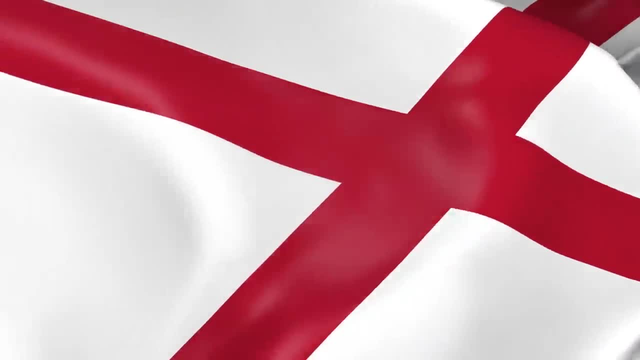 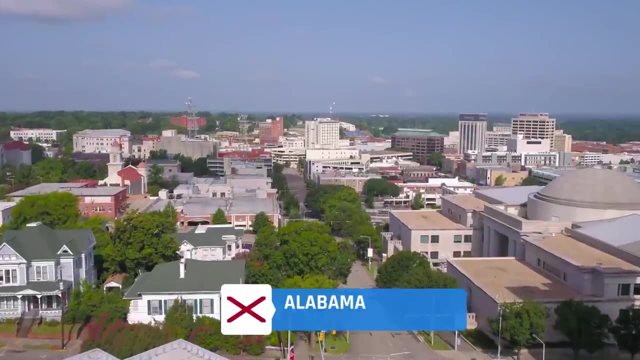 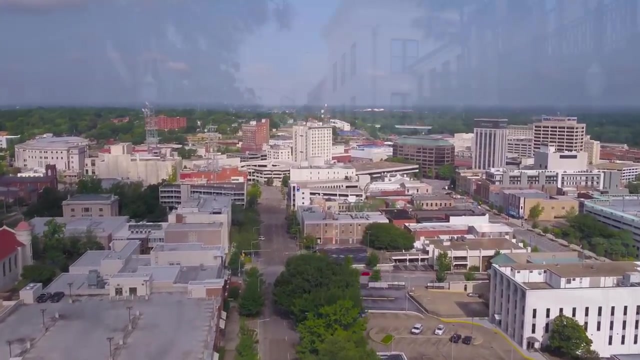 States. Number two: Alabama. the yellow jacket state comes in at number two And imagine that you're in a Southern state and stop typing. It's not the yellow jacket States, the yellow hammer state. How many of you froze the video, made a comment and now are just learning? I was joking.